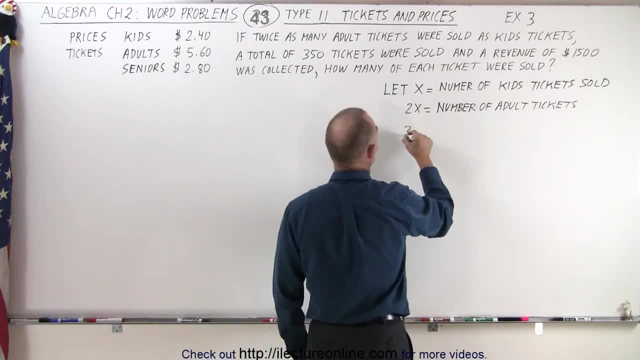 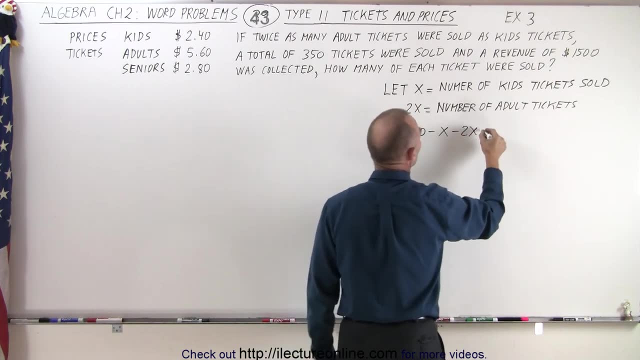 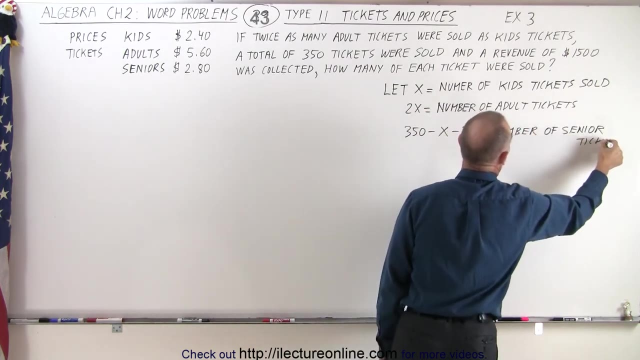 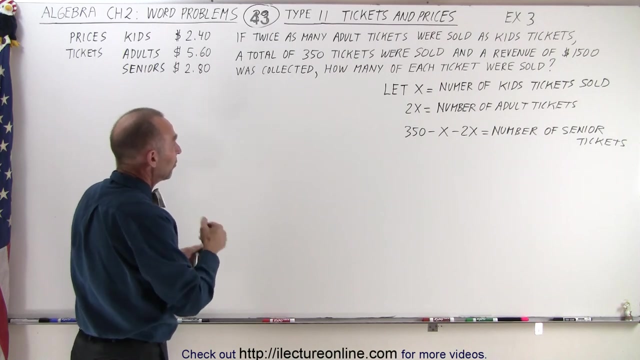 was a total of 350, which means 350 minus the number of tickets sold for kids, minus the number kids sold to adults, should equal the number of senior tickets. now to solve for x, we need to come up in an equation, and so the total revenue for kids plus the revenue for adults, plus the revenue. 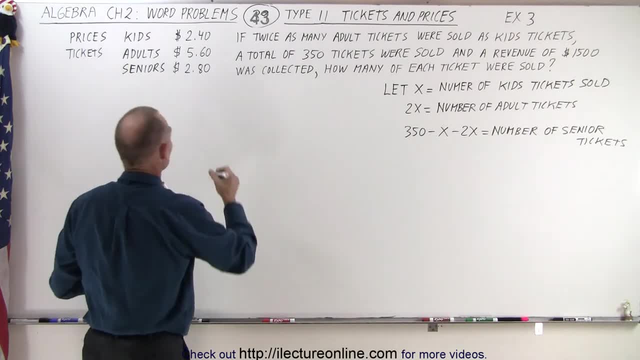 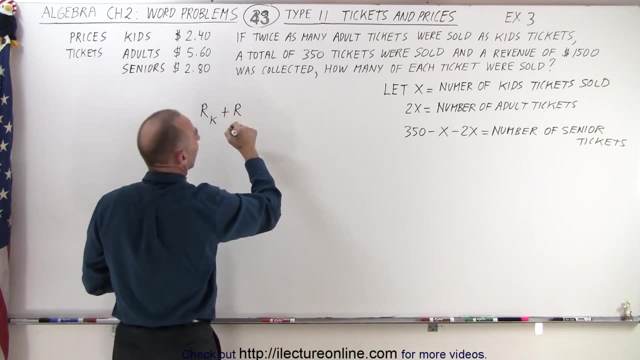 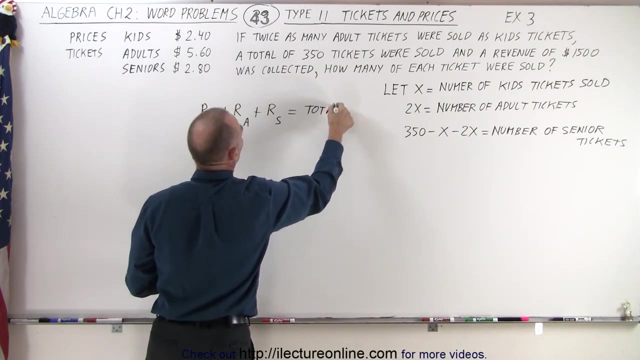 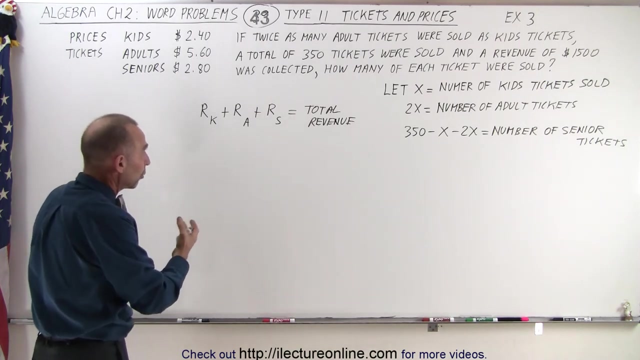 for seniors together should add up to the total revenue. so the revenue of the kids tickets plus the revenue of the adult tickets, plus the revenue of senior tickets must equal the total revenue. and there's our equation. we now simply have to turn into an algebraic equation. 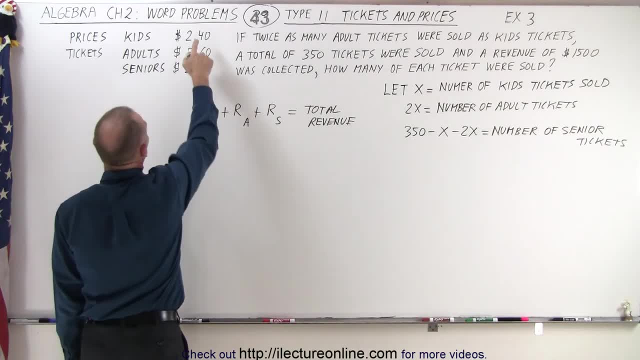 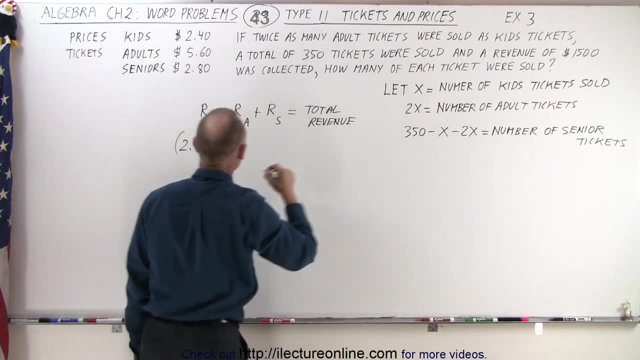 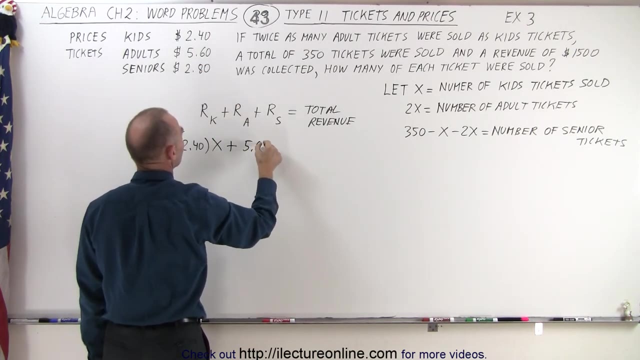 with x. so if we take the price of each ticket for kids, so i would be 240 times the number of kids tickets which was defined as x. we get the revenue for kids tickets plus the price for each adult ticket and we multiply that times the number of adult tickets. 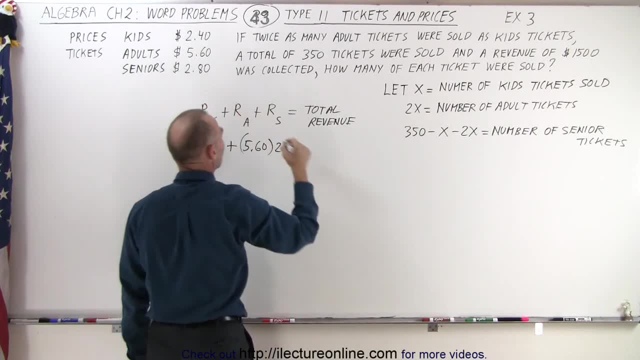 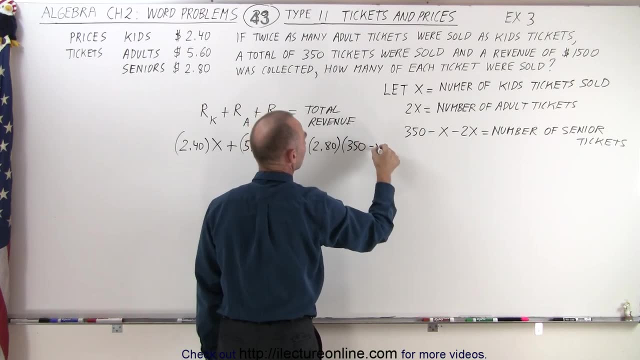 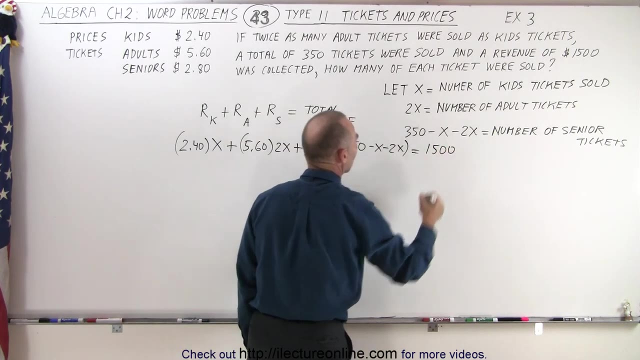 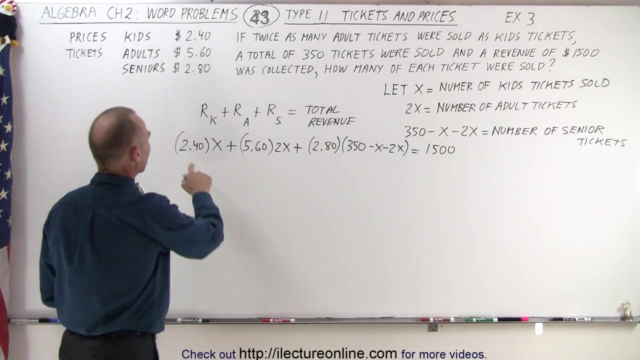 sold, which is 2x plus the price of senior tickets. times the number of senior tickets, that should add up to the total revenue, which in this case was fifteen hundred dollars. there we go. now we have an equation we can solve for x, so let's go ahead and simplify. first, we want to get rid of the decimal. 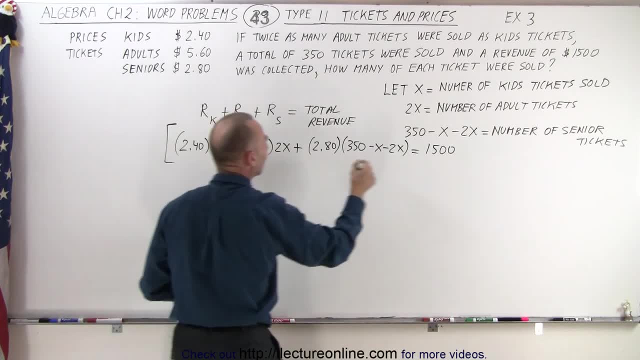 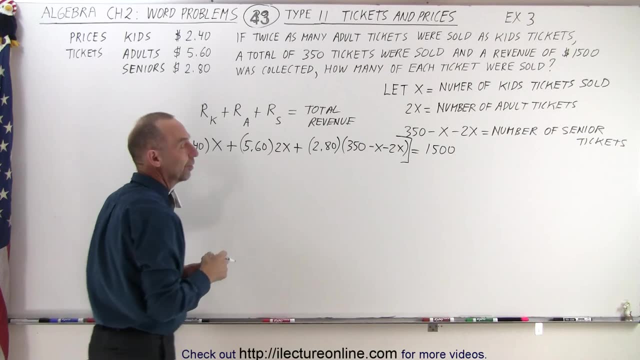 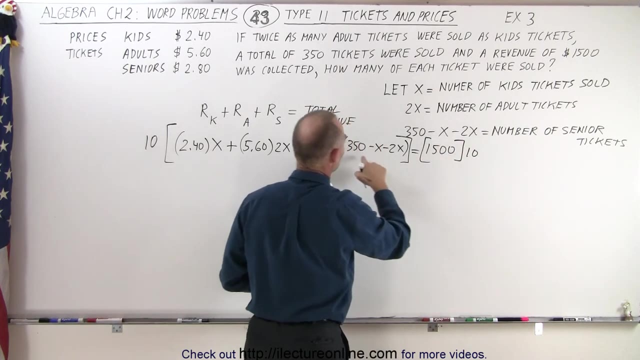 we can do that by multiplying both sides by ten. we don't have to do it by a hundred, because it's point two, zero, point two, point eight, zero, point six, zero, point four, zero. so multiplying by ten we'll get rid of the decimal. of course we need to do that to both sides and we can also combine what's. 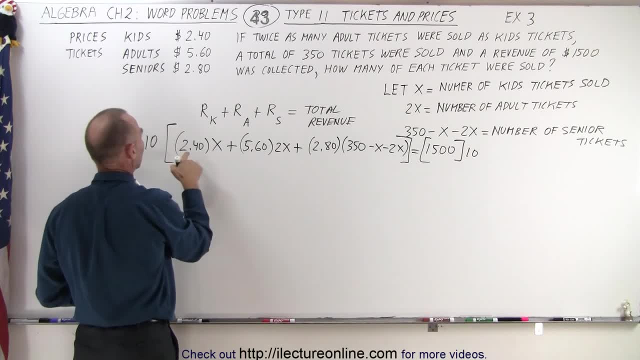 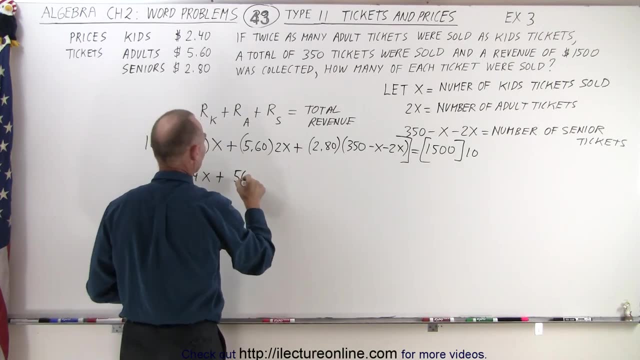 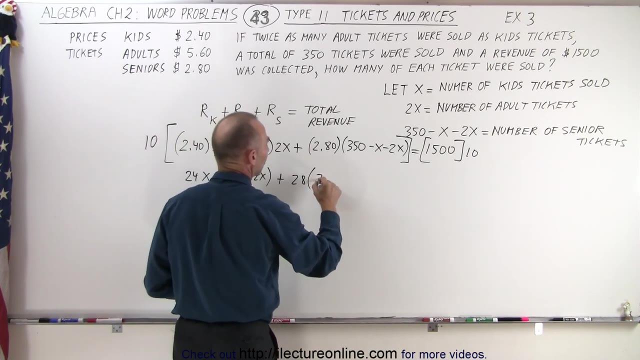 inside the parentheses here. so in this case, 10 times 2.4 gives us 24 times x. plus 10 times 5.6 is 56 times 2x plus that will become 28 times 350 minus 3x, minus x. minus 2x is minus 3x is equal to. 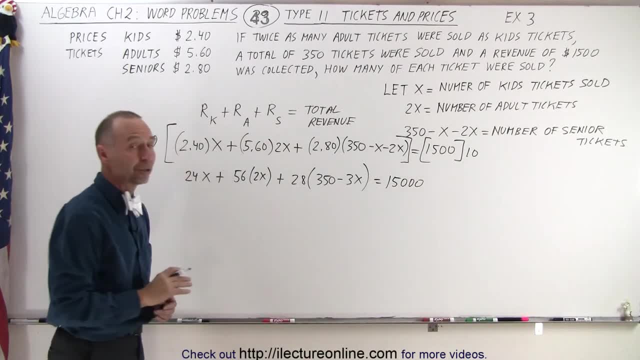 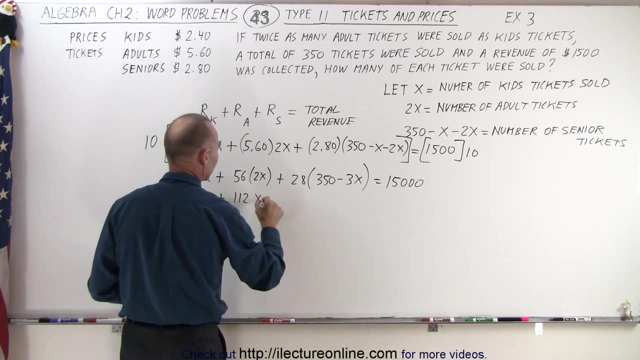 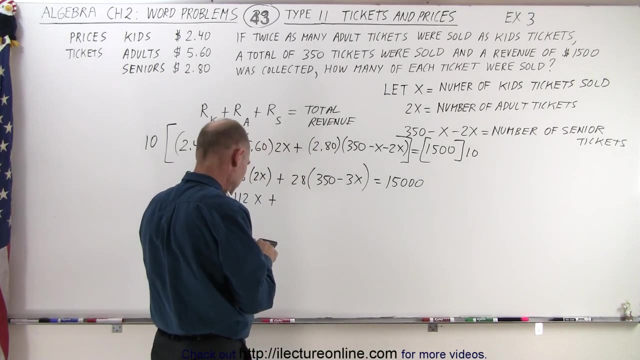 15 000.. now we need to get rid of all the parentheses, so this becomes 24 x plus 2 times 56, which is 112 x plus 28 times 350. well, let's get a calculator real quick: 28 times 350, that's 9800. 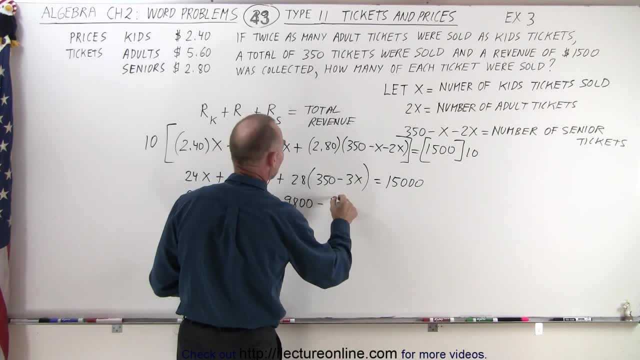 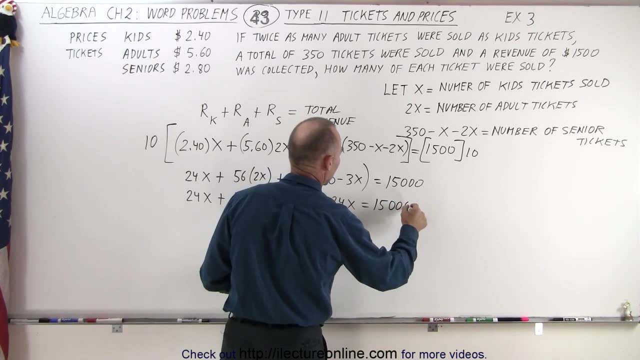 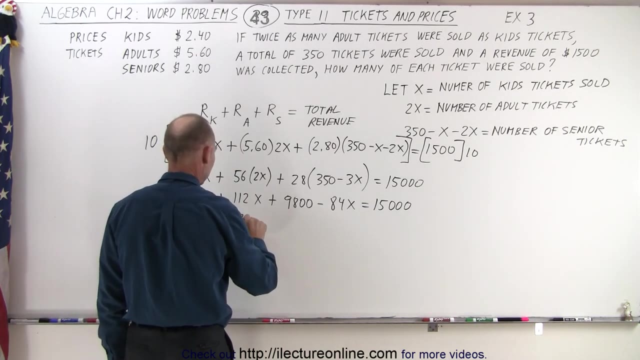 minus 3 times 28, that would be 84 x, that's 60, that's 24, that's correct, and that would be equal to 15 000.. now let's move all the x's to one side, while they're already there. move all the numbers to the other side. 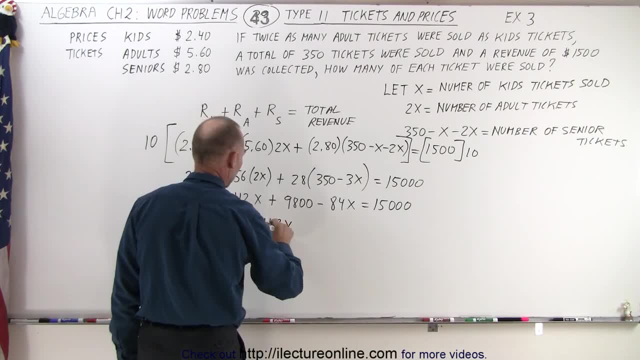 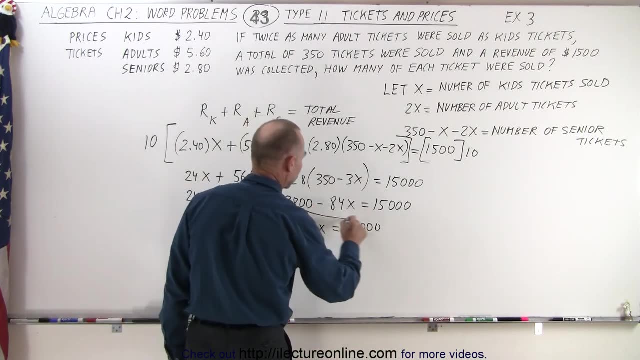 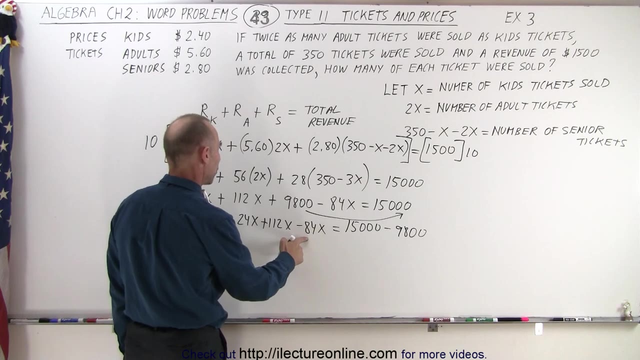 because this 24x plus 112x minus 84x is equal to 15 000 and we'll move the 9800 over here becomes minus 9800.. all right, combining like terms, 84, that would be 16, 12 that's four, that's 52, if i'm not. 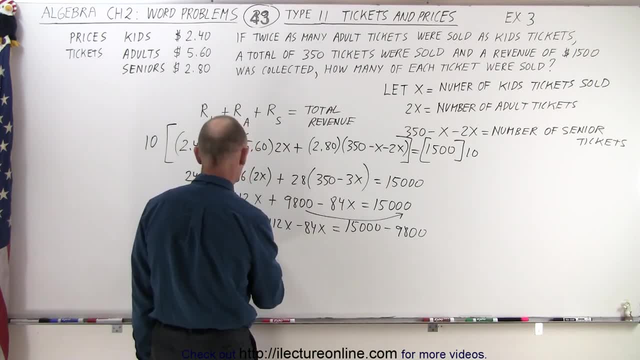 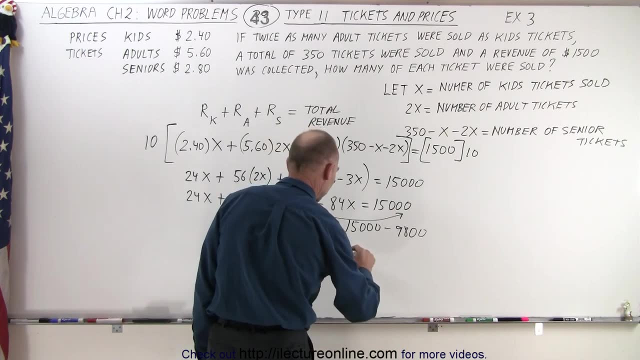 here. That's 12 plus 16 is 28,, 32,, 52x On the left side is equal to 15,000 minus 9,800, which is 5,200.. Divide both sides by 52, and we get x is equal to 100, even All right. going back to see, 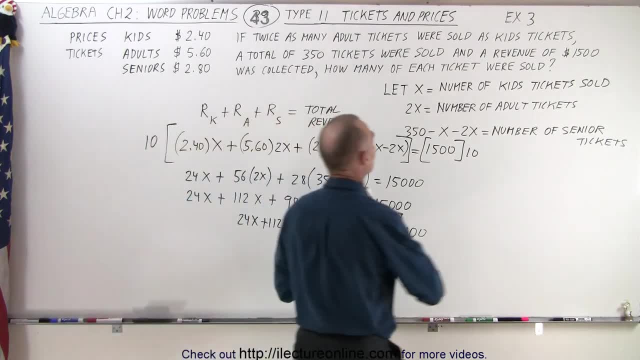 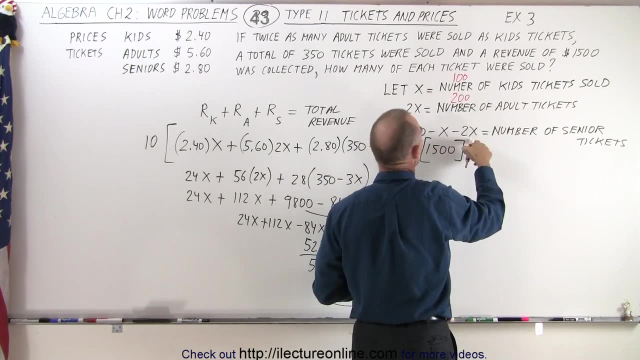 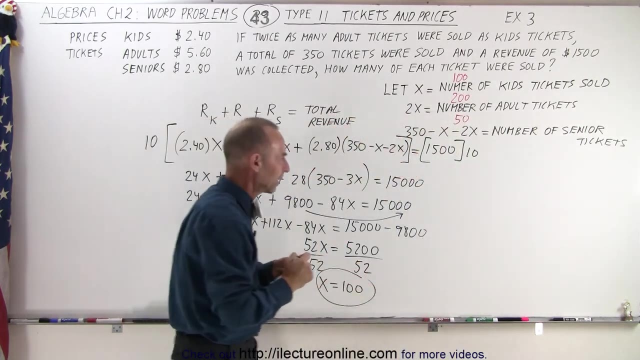 what x represents? it represents the number of kids tickets sold. That would be 100, twice as many adult tickets, which is 200, 350, minus the sum of the other two, which would be 50, and that gives us a total of 350 tickets. Now let's do a check, Make sure we have done this correctly. 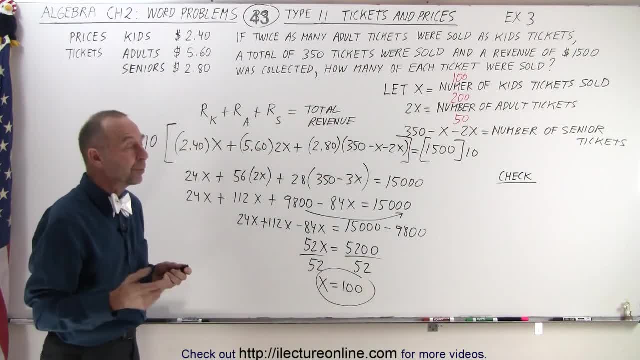 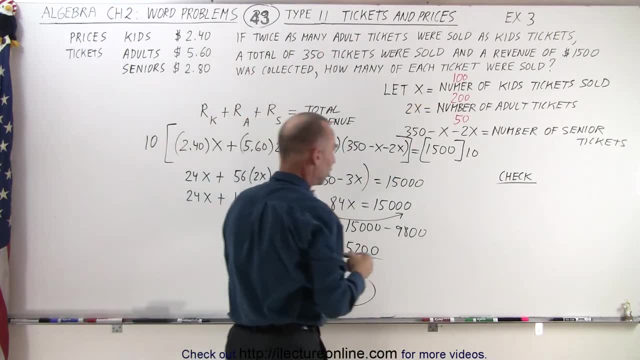 What we need to do now, of course, is figure out how much money was spent on each of the type of tickets. We have 100 tickets for the kids and they're 2,040 cents each. so for the kids we have. 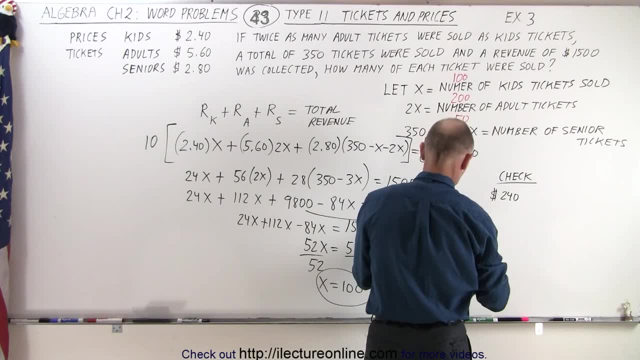 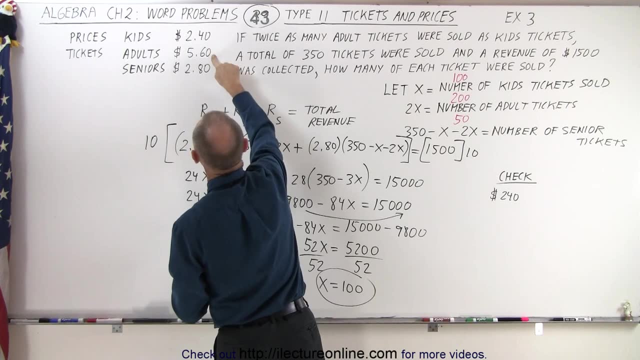 spent 240.. For the adults they're 200 each. I mean not 200 each. we sold 200 tickets and they're 560 each. so 100 of these is 560, double that that would be $1,120..